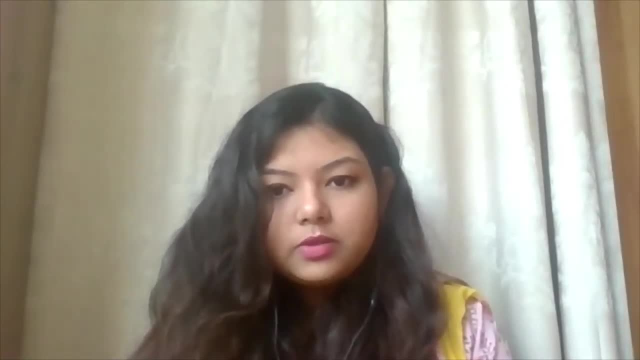 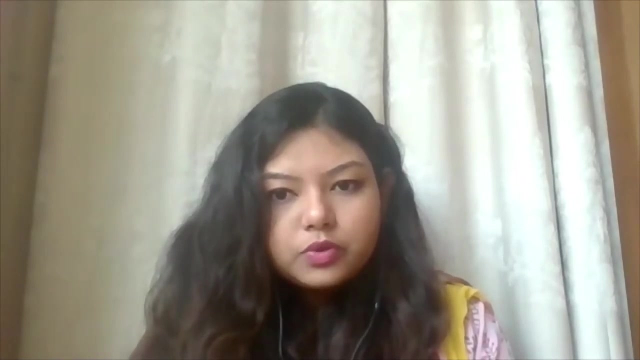 As-salamu alaykum everyone. I am Samira Sheikh, the Department of Electrical and Computer Engineering, ID number 1510049.. Today I am making this video for my lab final on neural network and fuzzy system session. I have chosen multilayer perceptron and now I am going to discuss about multilayer perceptron and I am going to analyze a code on that topic too. 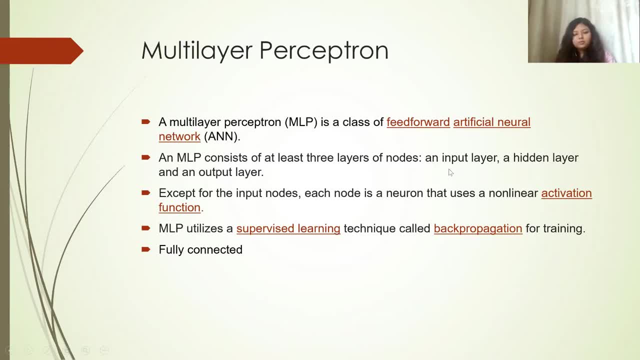 Now I am going to discuss about multilayer perceptron, what multilayer perceptron is and how the algorithm works. A multilayer perceptron is a class of feedforward artificial neural network, and multilayer perceptron consists of at least three layers of nodes and input layer, a hidden layer and an output layer. 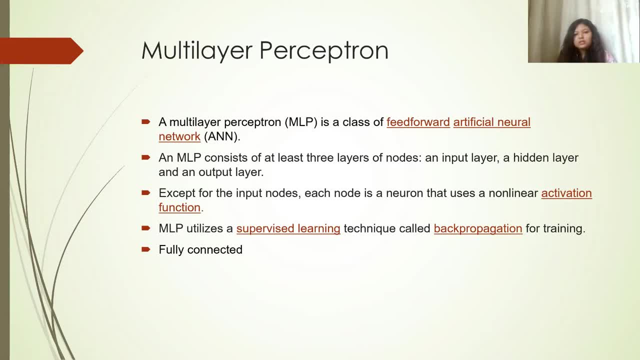 The input layer and hidden layer is constant, but we can change the size and number of hidden layer according to our requirement, Except for the input nodes, each node is a neuron that uses a nonlinear activation function. MLP utilizes a supervised learning technique called backpropagation for training. 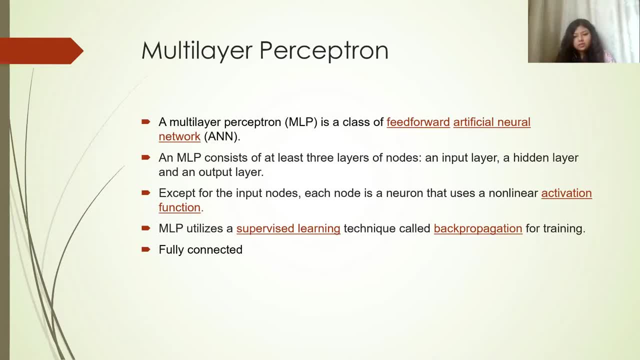 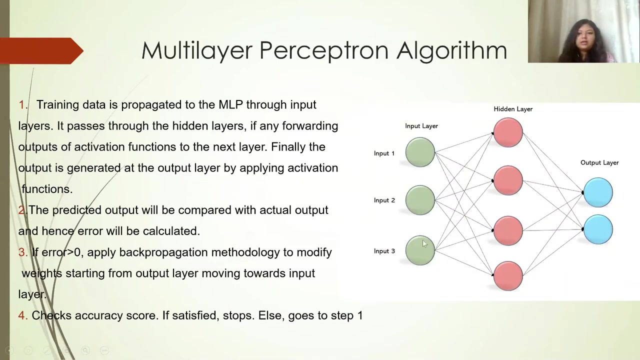 That means when our predicate value doesn't match with actual value, it changes the weight from the hidden layers and tries to learn better from the input data. And the most important thing is it is fully connected. I have provided an image here. We can see that the input layer, output layer and the hidden layer and how it is connected. 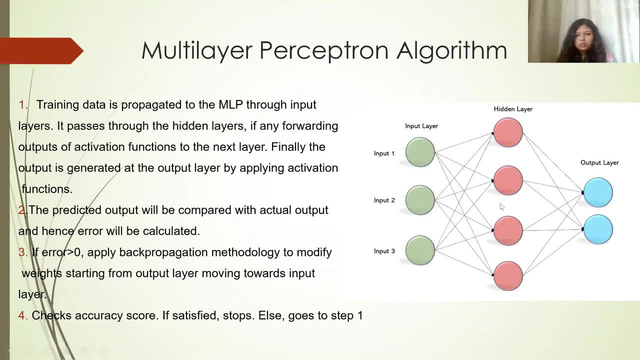 in multi-layer perceptron. So the multi-layer perceptron algorithm mainly propagates the input data through input layer and it passes through the hidden layer And then it passes through the output layer only when the activation function required for the output layer passes through the hidden layer. 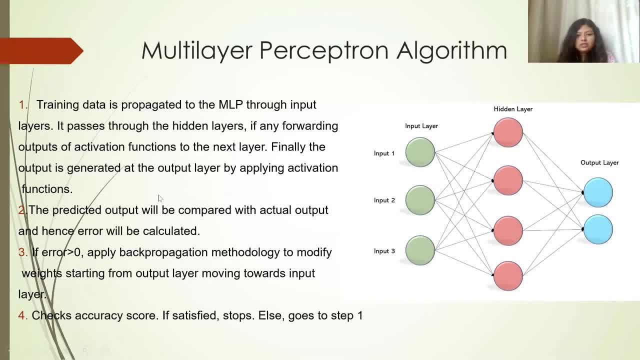 Then, finally, the output is generated at the output layer by applying activation functions. So what have I said before? The predicted output will be compared with actual output, and hence error will be calculated, And if error is greater than zero, backpropagation methodology is applied to modify weight starting. 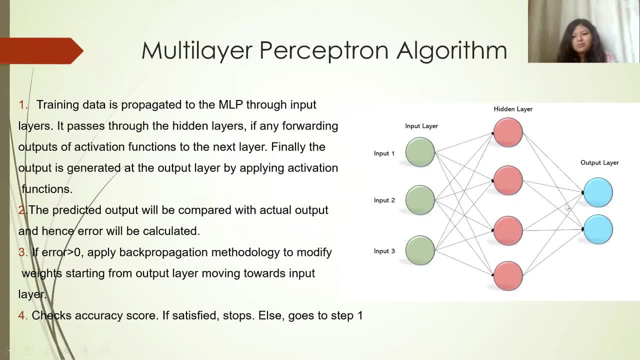 from the output layer moving towards the input layer. So it changes the weight by backpropagation, which means it starts from output layer and it backpropagates. And this is how the multi-layer perceptron algorithm works. And if the accuracy is satisfied, then the system is stopped. 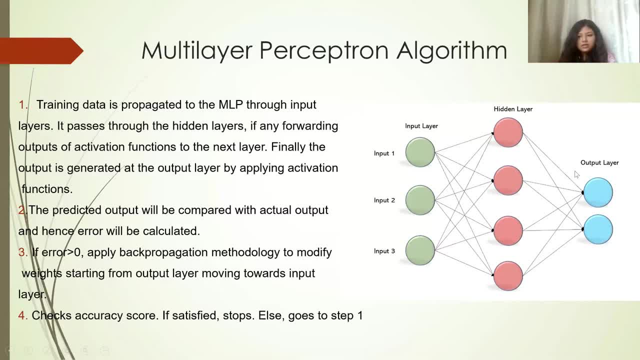 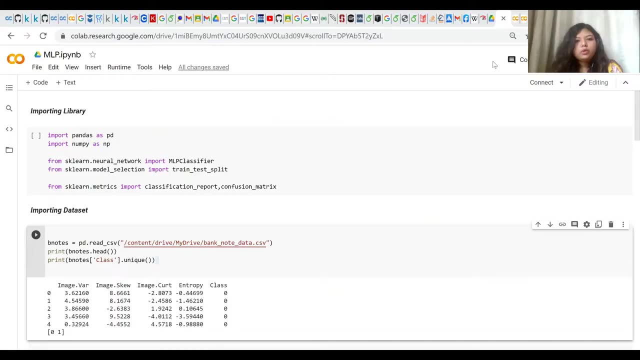 And if the accuracy does not satisfy the requirement, then the entire process goes back to step 1.. So this is how a multi-layer perceptron works theoretically. Now we are going to see a code on that algorithm. Thank you, So this is the code I am going to discuss on multi-layer perceptron. 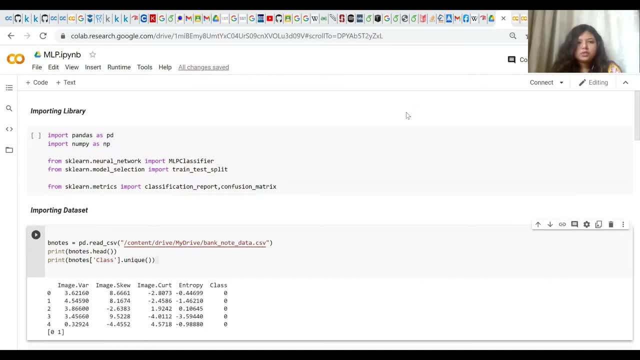 I have used Python And the environment I have used is Google Colaboratory. And here I have firstly imported some libraries. I have imported pandas as PD and numpy as NP And for the classification and training purposes I have imported MLP classifier from Espella. 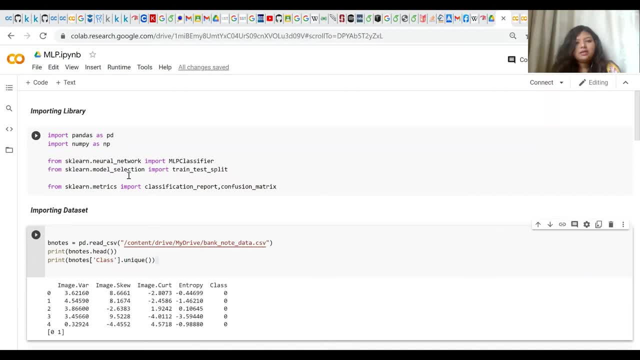 Neural Network and train test. split package from a skill and model selection for models evaluation. i have imported classification report and confusion matrix from a package from a skill and matrix test. next, i have imported the data set. i have imported the data set- a banknote data- and read the data. and read the data set in bnos and here. 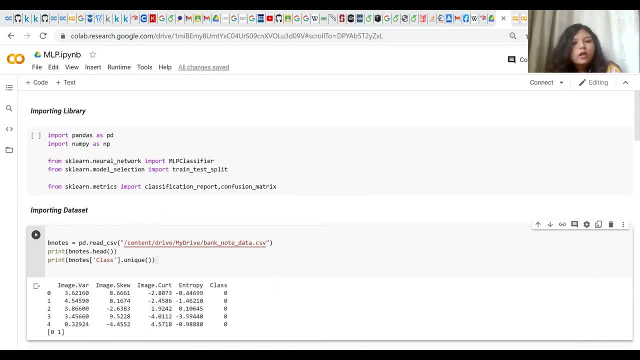 the banknote data is available in kegel and i have checked the data set and the attributes of the data set. we can check there. there are is five attributes- var, skew part and entropy and class, and we are going to train and test the data on the basis of. 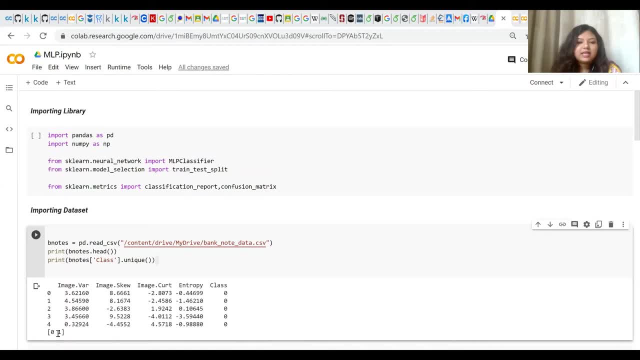 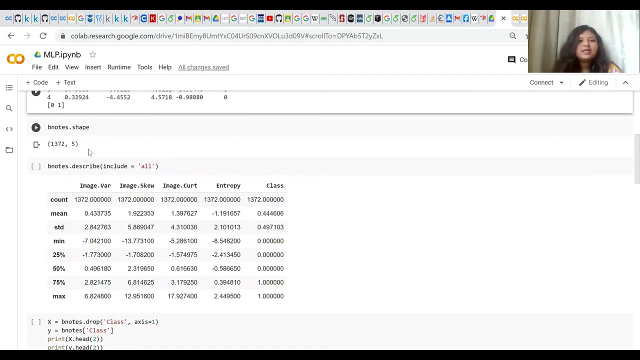 class. so we have checked the unique data in class. this is by bnotclassunique command and the unique data in class is zero and one, so this would be a binary classification. and we have checked the shape of the data set by bnoteshape command and we can see that the data in the data set has 100 1372. 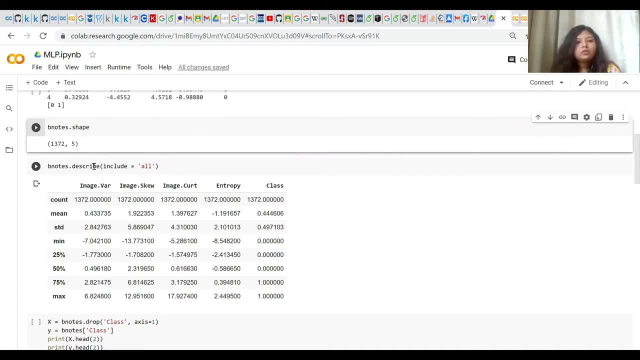 identity and five address fields and by bnotedescribe input equal to all command. we have checked if there is any null value in the data set or we need to entry any value in the data set manually. we can see that there is no such values in the data set. 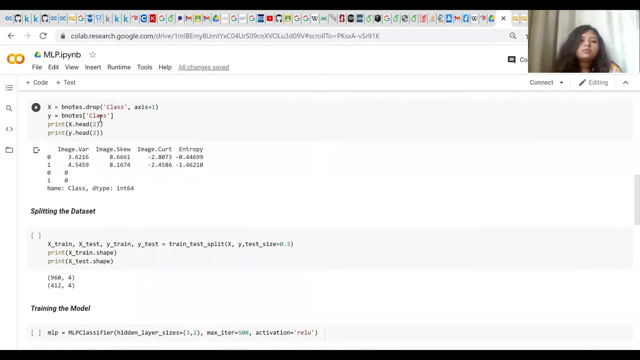 in the next window. we have created two data set here. one contains the other four attributes and the another data set contains only that plus attribute, because we need to train and test the data on the basis of class. so we have simply, by drop function, we have simply dropped the class attribute from the data set. 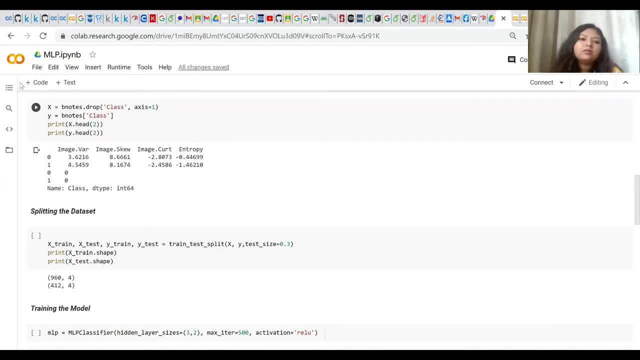 here and we put it in x variable and the class is in y. so we have checked if our command is done successfully. we can see that uh. for the first two rows we can see that there is no class and in other uh two we can see that uh. 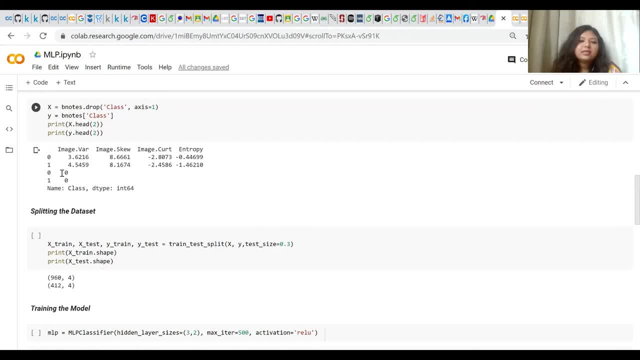 there is no class and in other uh two we can see that that there is two data from class attributes. next we need to split the data set. for splitting the data set, we have used the train test split and then we have defined the test size as point three. that means that our test size 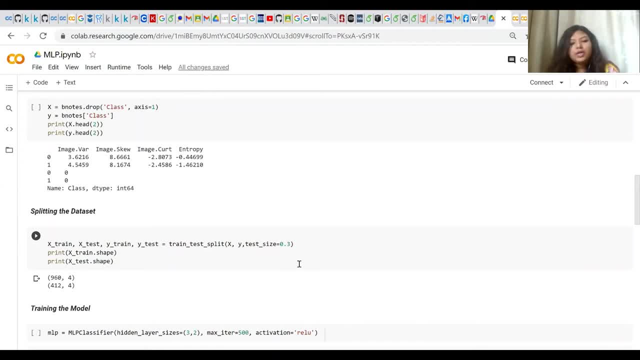 would be 30% of the data set and our training set would be 70% of the data set. it they will have recreate the shape of the training and test Popup. here we can see that the training dasid have 960 identity of having four attributes and 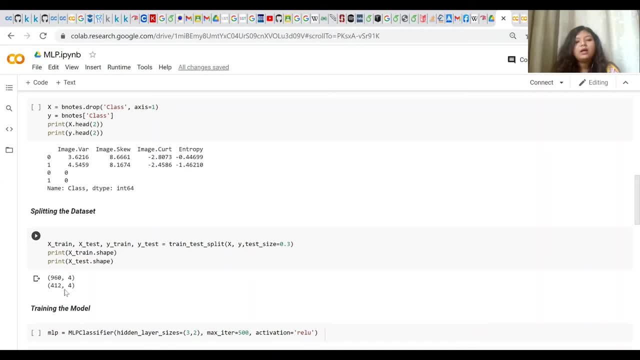 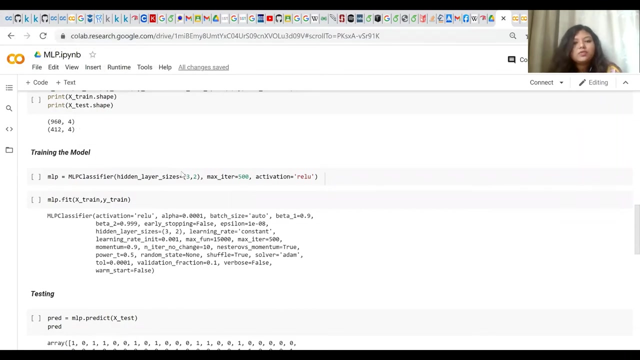 the testing that, as I have 412 identity and four Publix and we have dropped the class from the that. we have dropped the class attribute from class, the X train and X from X. now we are going to train the model for training the model we have used. MLP classifier: the hidden layer, the size of the hidden. 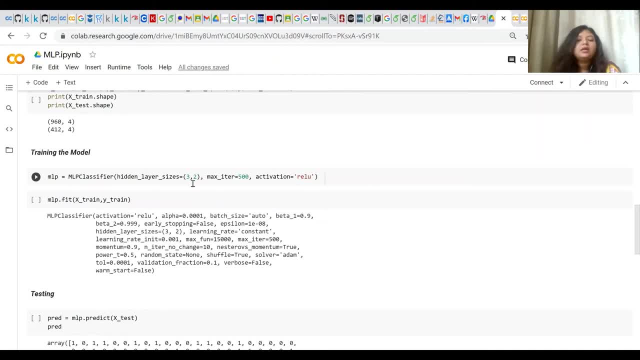 layer is 3 and the size of the hidden layer is 2 and more of the hidden layer is respectively 3 and 2, the max iteration is defined as 500 and the activation function is used as ReLU. ReLU means rectified linear image in by. 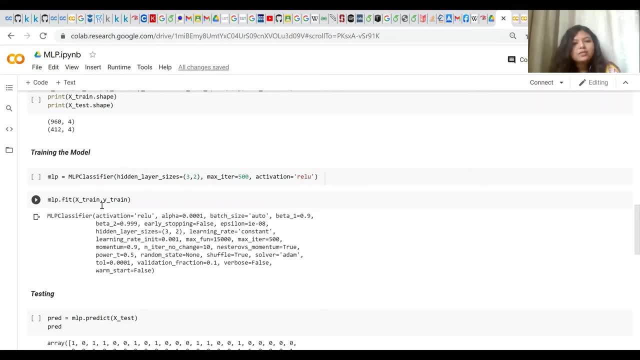 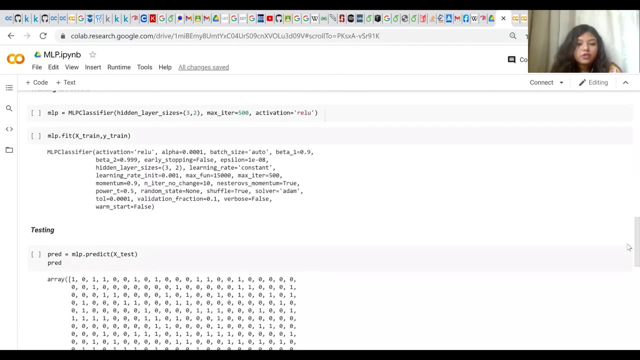 MLPfit. we have fit the training data- X train, Y train- in the material perception model and then we have, after finishing, 500 iteration of training. we have tested the data and we can see that the training data has been tested and we can see that the training data has been. 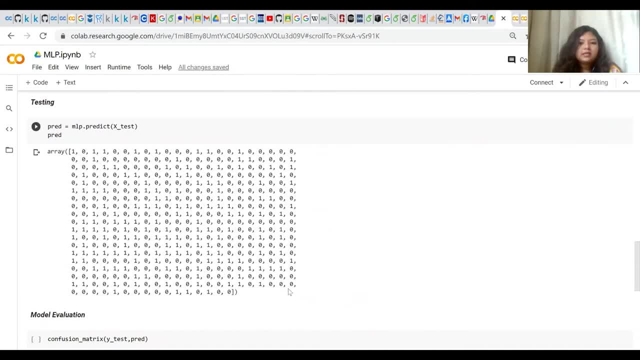 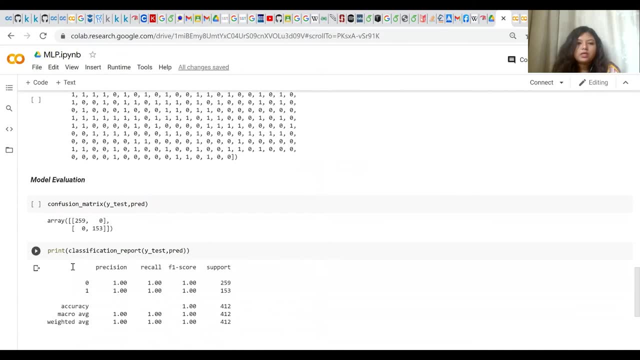 there the prediction of the material perception. here and after that we have evaluated model so we can see how the more how the material perception does for our banknote data set and from the confusion matrix we can see that our case you know. from the conclusion matrix we can see that it has correctly predicted 259, truly positive. 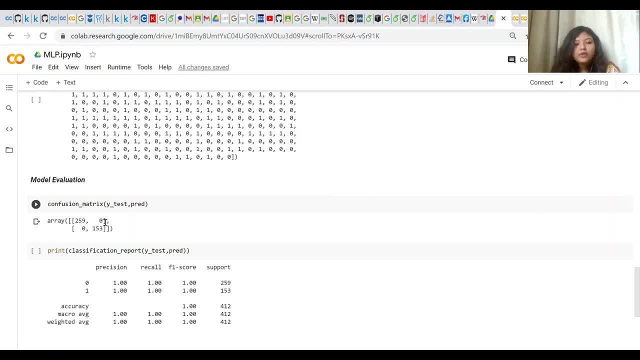 and 153 truly negative. so there is no values in false positive and false negative, so that our model has done good with the data set and it has learned perfectly from the data set. and by printing the classification report we are checking the precision, recall F1 score and the accuracy of the model. we 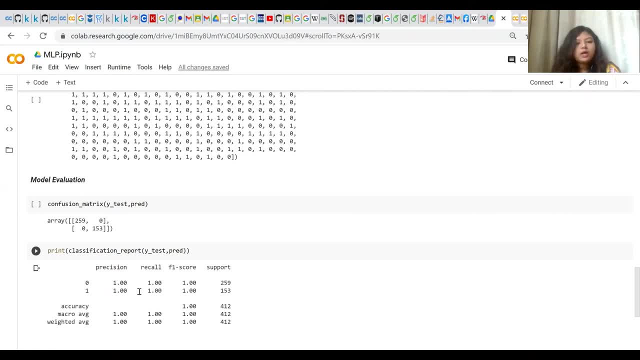 can see that for each zeros and once our position is one, recall is one, F1 score is one and- and here the support for 0s. there there are two hundred and fifty nine zeros and 153 1, which have been perfectly classified and the accuracy. 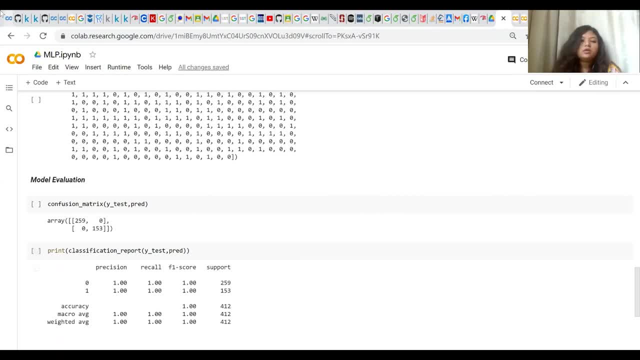 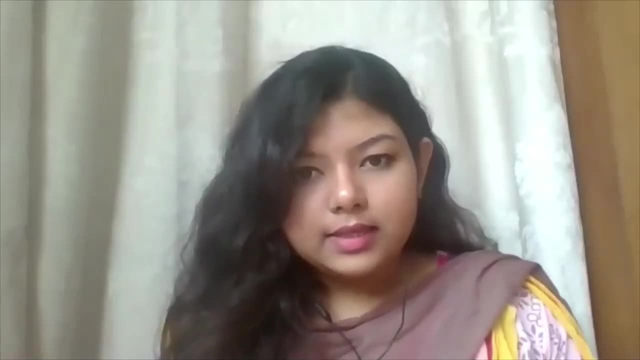 is one for four hundred and twelve data chosen randomly from the data set so that we can say that our model has predicted perfectly and it has been trained perfectly and it is compatible with the data set we have used. Thank you everyone for being with me till now. Assalamu Alaikum.